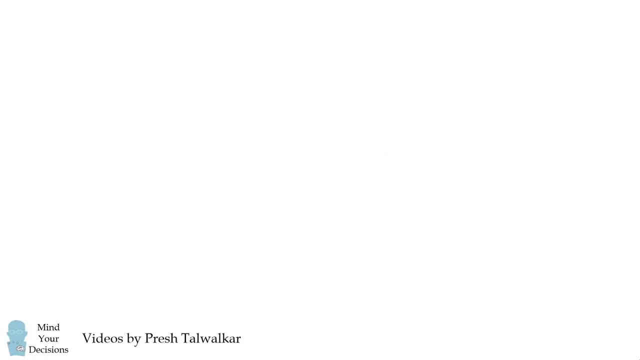 Mind your decisions. I'm Presh Talwalkar. Start with a semicircle From the upper right corner. carefully fold a circular segment until it just touches the diameter and divides the diameter into lengths of four and two. The question is: what is the length of the folded line? 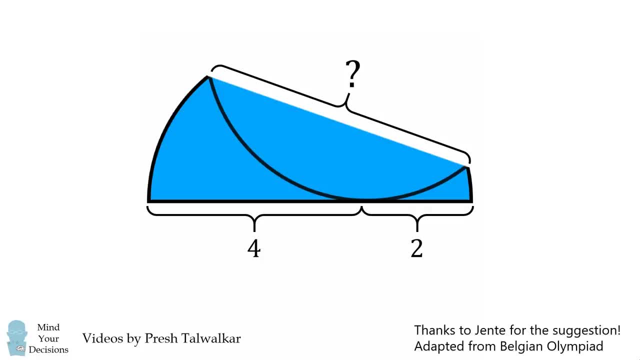 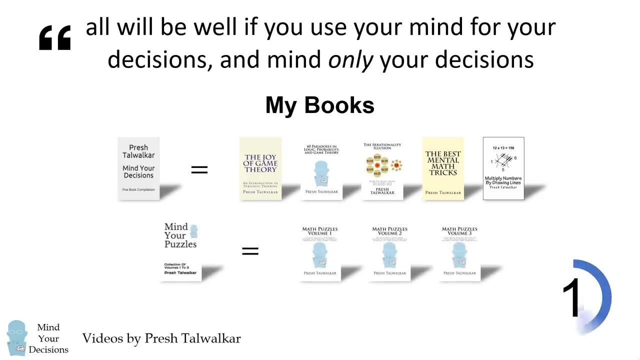 I thank Yenta for the suggestion. The problem is adapted from a Belgian mathematical Olympiad. Pause the video if you'd like to give this problem a try and, when you're ready, keep watching to learn how to solve this problem. To solve this problem, we must use the little gray cells. 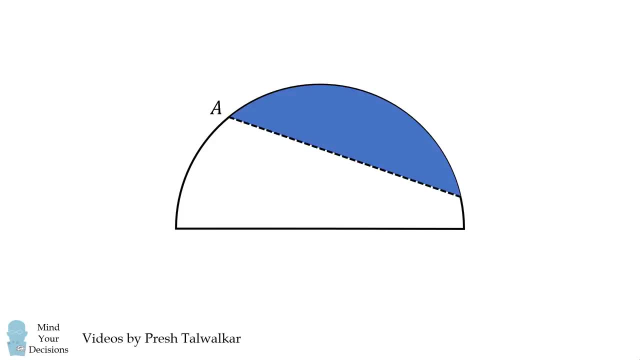 We start with a circular segment that is reflected about line AB. The resulting circular segment is tangent at point T and divides the diameter into lengths of four and two. The entire diameter will have a length equal to six. Label the center of the semicircle as P. The radius of the semicircle will be one-half its 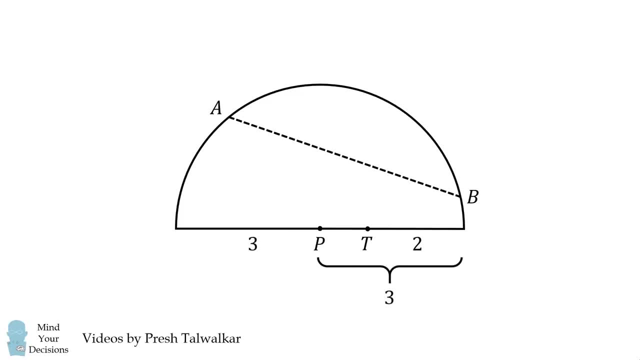 diameter and therefore it will be equal to three. Consequently, PT has a length equal to one. Now consider the reflected or folded circular segment. Let's draw the circle containing the circular segment, Because the original circular segment belonged to a semicircle of radius three. 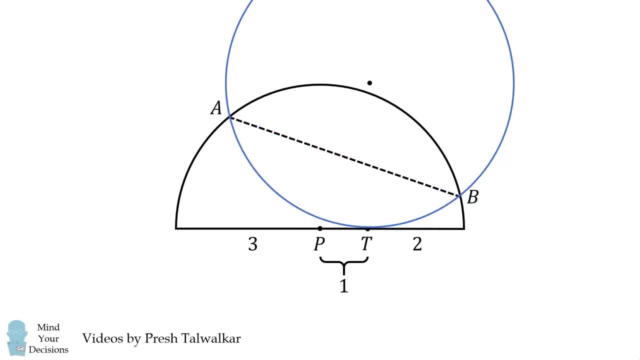 the resulting circle will also have a radius equal to three. Furthermore, the center of this circle will exactly be the image of P about line segment AB. You can see this because both are equidistant from point A and B. Now pick the line segment AB and the area with the original circular segment. 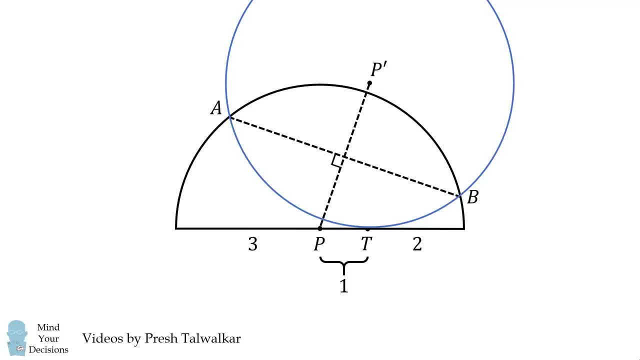 and B, and there is symmetry about line segment AB. If we construct P, prime T, it will be perpendicular to this diameter and it will have a length equal to 3.. We can therefore focus on just this right triangle. We can calculate the length of the hypotenuse using the Gogu theorem and we get. the distance between the two centers is equal to the.